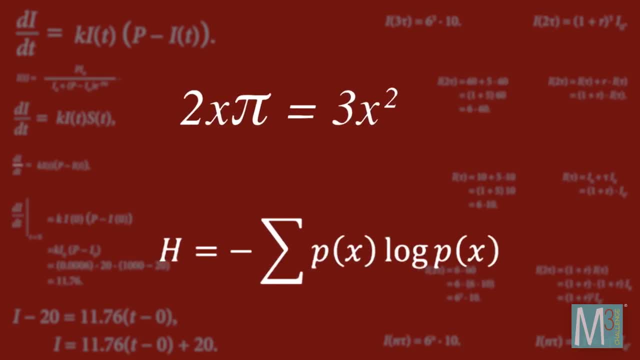 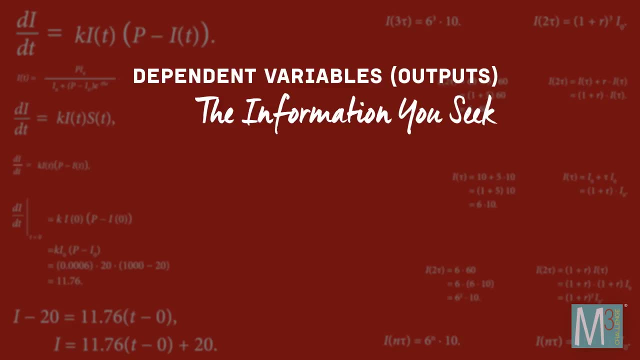 them, The variables you need to develop your solution, come from the perspective of the problem statement. Dependent variables are often called outputs. They represent the information you seek. Independent variables, also known as inputs, represent quantities. you know the value of, but may change. Fixed model parameters represent constants: those quantities that 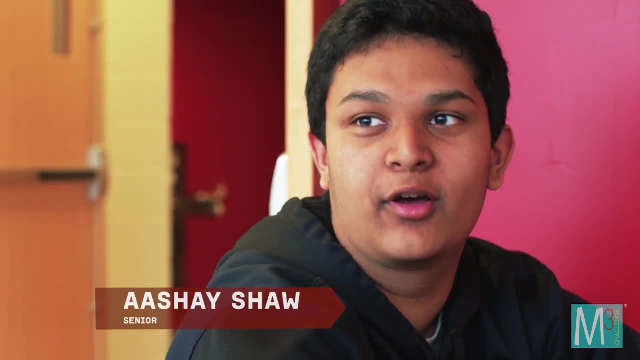 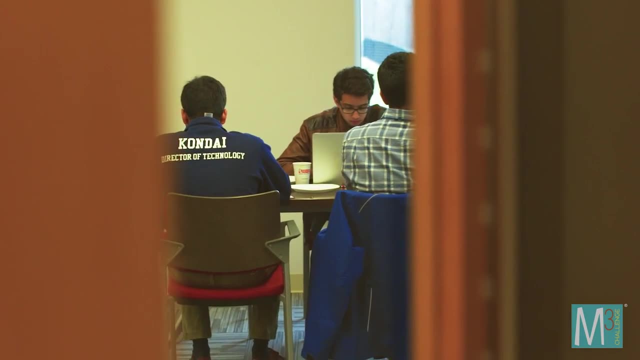 remain the same. You have to figure out what you know and what you don't know in your model, And whatever you don't know is what you need to define. Once you figure out what you don't know and what you do know, then you can define your variables. Let's say you're a painter. 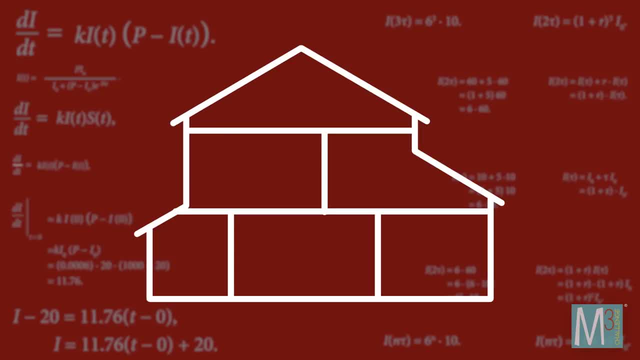 Before you start a job, you'll need some information. You'll need information that will help you determine how many gallons of paint to buy for each room of the house. You can take measurements to calculate the size of each room. Those are your independent variables, or inputs. You also know how many square feet a particular 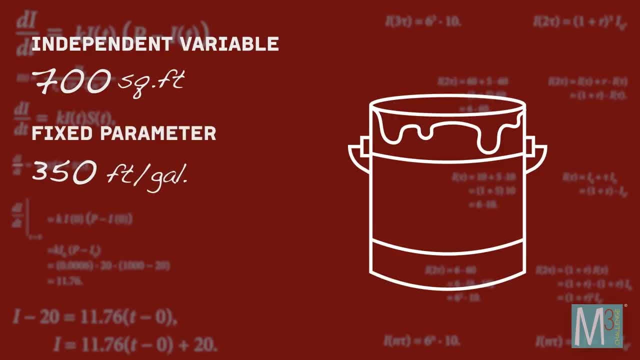 brand of paint will cover. That's a fixed parameter. The only thing you don't know is the volume of paint you'll need. so that's the dependent variable or output you seek. Once you've figured that out, you're well on your way to finding a solution In this. 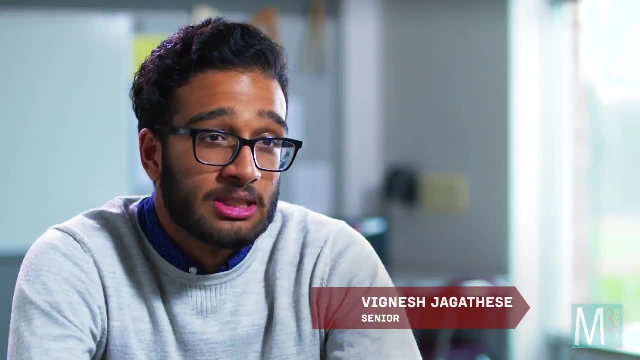 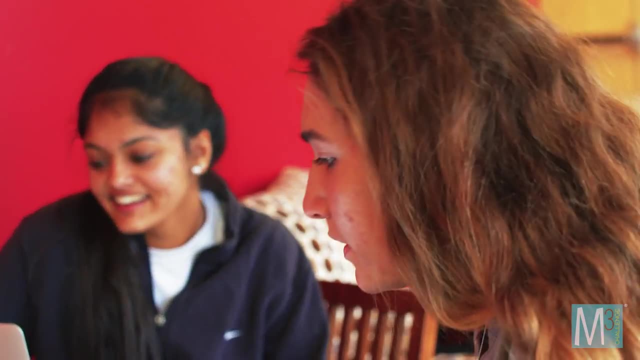 case, we'll use a different formula to define the volume of paint we'll need. It's a variable by two gallons of paint. when we listed out all the possible things that could change, the ones that really could be irrelevant went to assumptions, but the ones that we deemed extremely, extremely relevant went into our variables most. 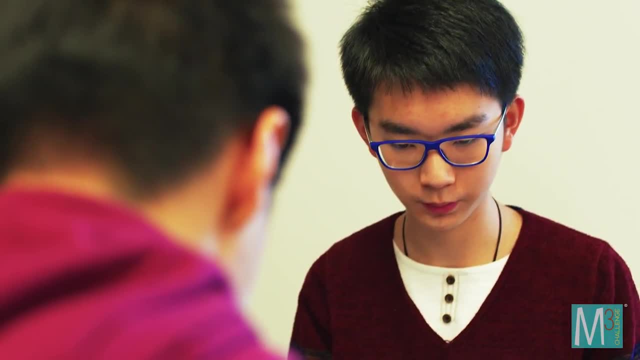 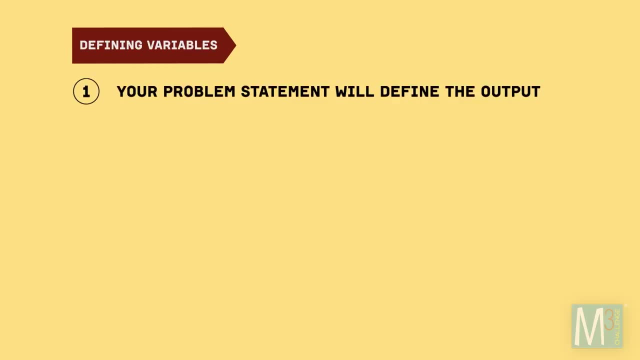 important part about determining your variables is understanding the problem. if you understand the problem, the variables are just right there in front of you. here are some things to remember when defining variables. your problem statement will define the output or dependent variable of your model. your initial brainstorming should give you the clues to define your independent 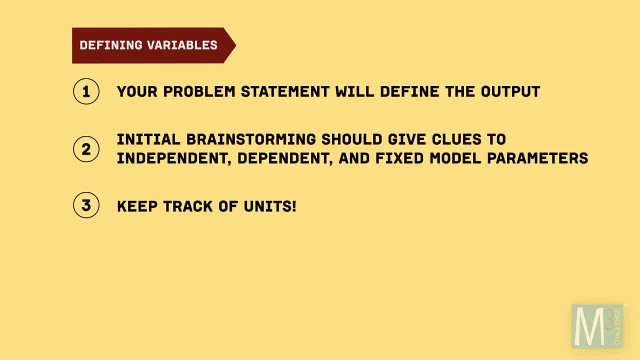 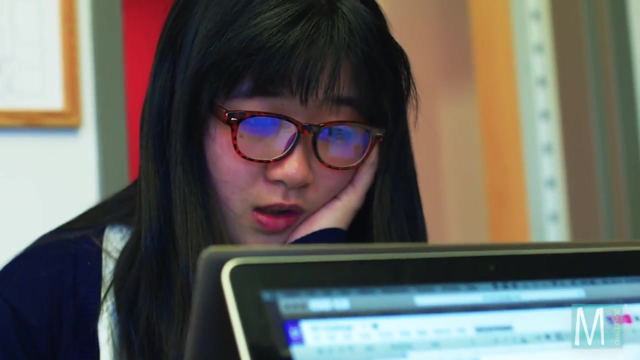 dependent and fixed model parameters. keep track of the units of measurement you're using because they can reveal relationships between variables. you may need to do additional research or make new assumptions to find values or parameters. sub models or multiple models may be needed to reveal certain model input. your problem definition, combined with your assumptions, will help you find.